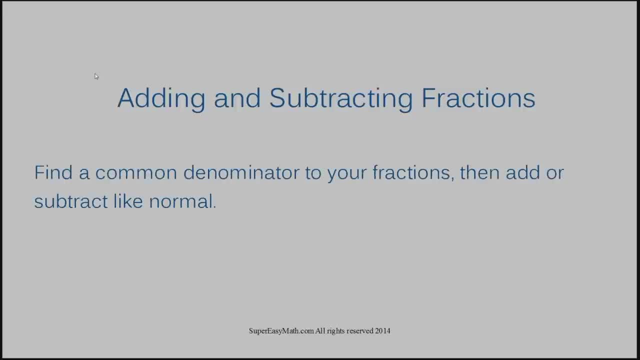 Adding and subtracting fractions. When adding and subtracting fractions you want to remember to find the common denominator to your fraction then add or subtract like normal. Let's look at example number one. Example number one. We already have common denominators for this example so adding is going to be pretty easy. When adding fractions all you do is add the numerators. 1 plus 5 is 6. Your denominators always stay the same. This answer can be simplified so that means I can divide my numerator and denominator. by something that is the same number. They're both even so whenever your numerator and denominator are both even that means 2 can always go into both of them. I'm going to divide by 2. 6 divided by 2 is 3 and 14 divided by 2 is 7. 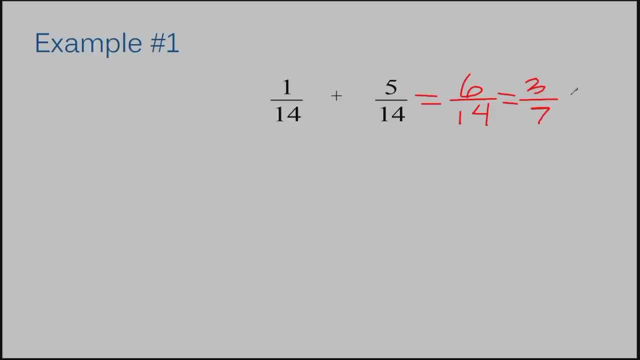 There's nothing that can go into both 3 and 7 so 3 sevenths is my final number. 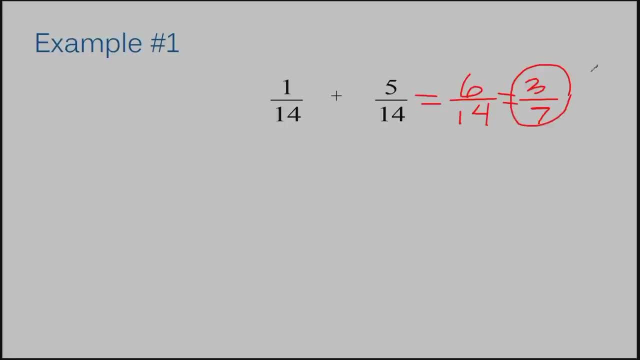 Let's move on to example number 2. Example number 2. For this example our denominators are not the same so we need to make them the same before we can add. I'll show you a trick that always works when you need to get a common denominator. Whenever you multiply your two denominators together that will always always always give you a common denominator. The only thing is sometimes your denominator may be kind of large if you do that. If you do that you're going to have a common denominator. may not be the least common denominator okay but it will work what will happen is you'll just have to simplify your answer at the end so let's try multiplying our denominators together to get a common denominator so I'm going to rewrite both of these numbers directly below but with the denominator of 80 now the steps that I take to go from the 8 to the 10 what I did was multiply by 10 remember that's what we did so if I multiply something on the bottom of my fraction if I multiply the denominator by anything I must multiply the numerator by the exact same number that's the only way I'm going to keep the value the same I talk about this in my equivalent fractions video if you are not so sure of how to keep 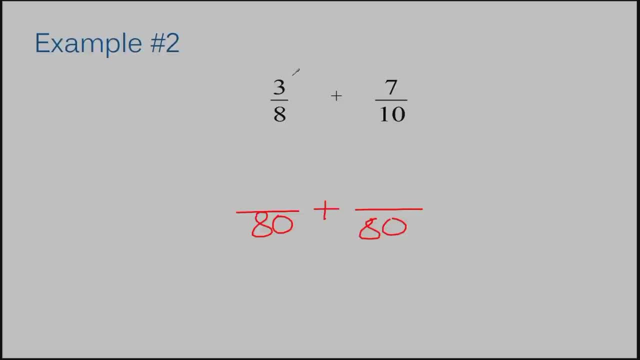 your fractions equivalent you can check out that video and it'll give you a better understanding but 3 times 10 is going to be 30 and the same thing happens over here we multiplied the 10 by 8 to get this 80 so I have to multiply my numerator also by 8 so 7 times 8 so I have to multiply my numerator also by 8 so 7 times 8 so I have to multiply my numerator also by 8 so 7 times 8 is 56 now I can add if you remember before the denominator always stays the same so I went ahead and wrote it in now I'm going to add my numerators I have 30 plus 56 that's 86 okay we have a problem here and that is my numerator is larger than my denominator so to fix that what I need to do is to divide the denominator into the numerator that set up would look like this when you subtract you're going to get a remainder at the end so like you're going to subtract and you would end up with a 6 down here now I can do this in my head and I think you probably can too what I'm going to do is I'm going to make my whole number a 1 and then I'm going to subtract in my denominator here and I'm going to add 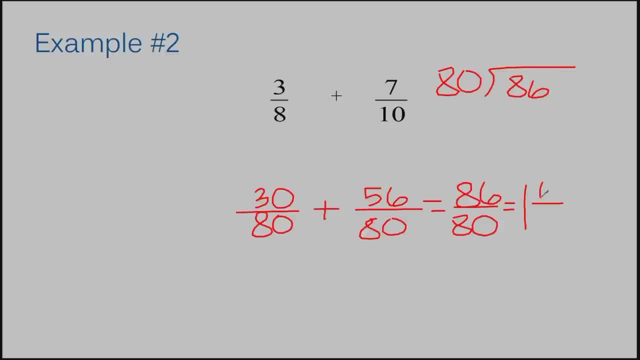 and subtract in my denominator here in the denominator and that's going to be 86 now let's say 86 goes into 86 one time and then there's six leftover you see 86 is only six more than the 80 so the extra that you had left over comes here and the denominator remains the same so that's the same thing that would have happened up here really I just did this step in my head that would have been 80 going into 86 is 1 and that's 80 and when I subtract I get my six so the numerator came from but I basically did this whole process in my head to get this the only problem with this answer is the 6 and the 80 can be simplified they're both even so I know at least 2 can go in them so I'm going to rewrite this answer as 1 and I'm dividing the numerator and denominator by 2 and I get 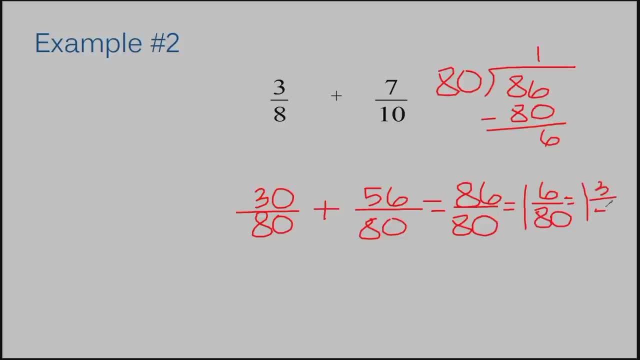 3 over 40 nothing can go into both 3 and 40 so 1 and 3 40th is my final answer 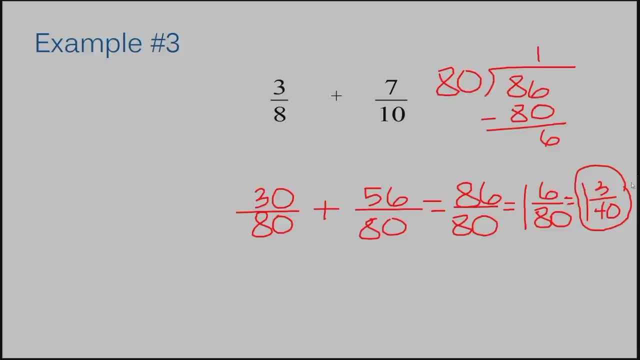 let's move on to example number 3 example number 3 I have 3 7th plus 20 over 35 I need to get a common denominator sometimes when you're dealing with fractions one of your fractions will already have a denominator that the other fraction 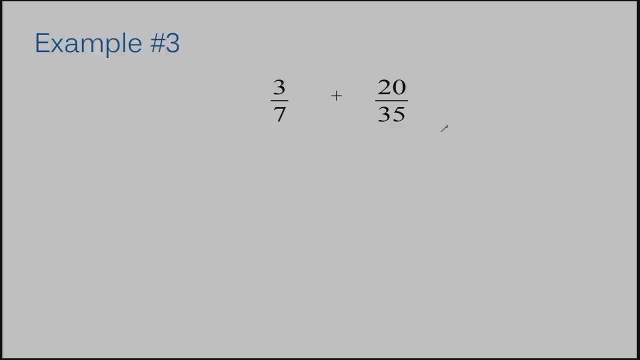 can go into meaning you may not have to change both fractions in this case 7 can evenly go into 35 so I know that this fraction doesn't need to change I've rewritten it right below the reason it doesn't need to change is because I can make this other fraction over here have a denominator of 35 but I have to ask myself what did I multiply the 7 by to get the 35 and the answer is 5 so I multiply the denominator by 5 so that means I must also multiply my numerator by 5 so 3 times 5 is 15 so now I can add my 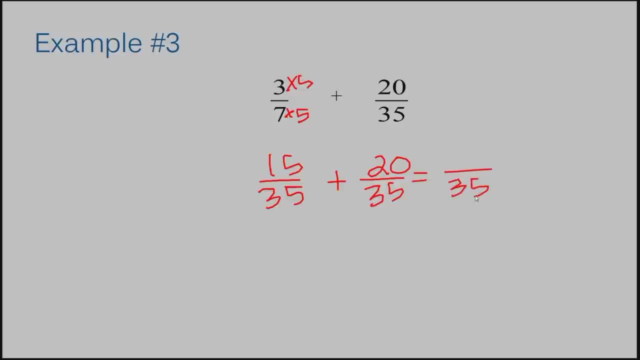 denominators remain the same 15 plus 20 is 35 we have the same number as our numerator and denominator whenever we have that that always means that our answer is just plain old 1 so the final 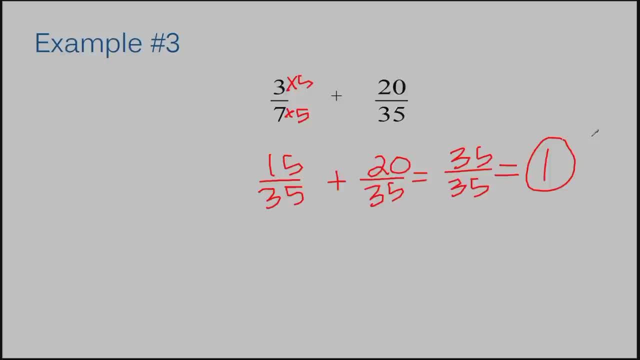 answer for example number 3 is 1 let's move on to example number 4 now we have subtraction we still have the same rule we still need to get common denominators for this example that 15 works as the denominator because 5 can go into 15 so this side I know is fine I'm going to leave it alone and just rewrite it. 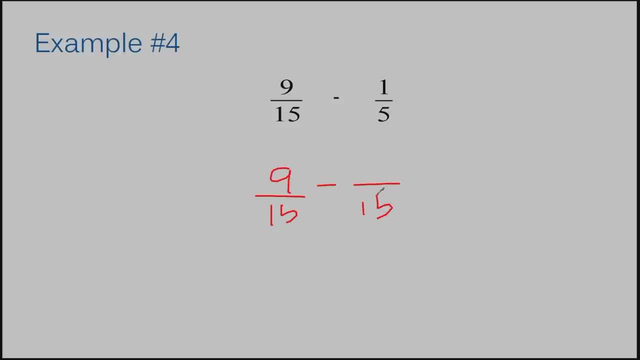 I'm going to make this denominator a 15. Now I ask myself, how many times does 5 go into 15? It goes into it three times, so that means 5 times 3 is what gave me the 15. I need to multiply 3 on the top as well. So 1 times 3 is what my numerator is made from. 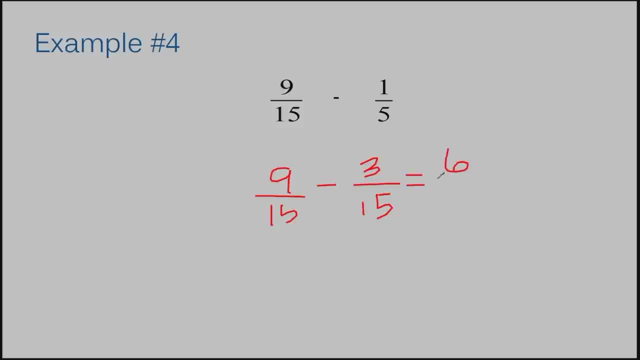 So 9 minus 3 is 6. The denominator remains the same. Is there a number that can go into both 6 and 15? Yes, that would be 3. So I'm simplifying now. 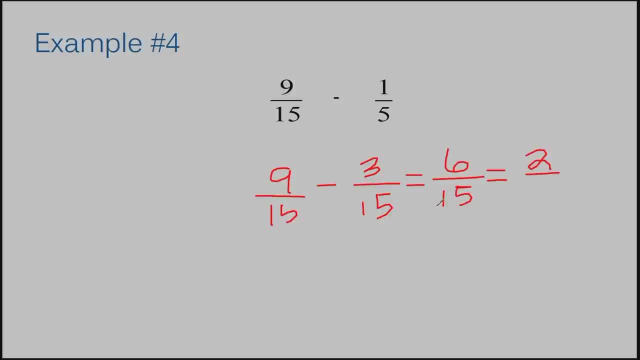 6 divided by 3 is 2. 15 divided by 3 is 5. 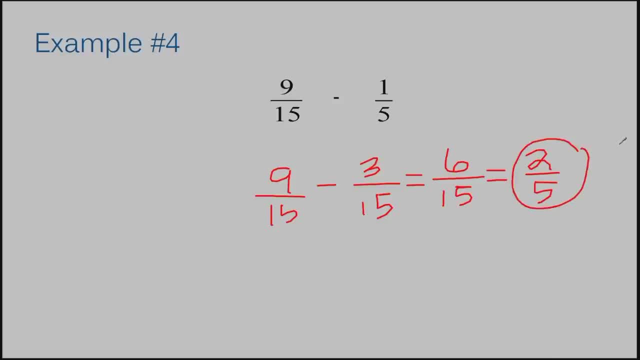 So my final answer to example number 4 is 2 fifths. Example number 5. I need to get a common denominator here. 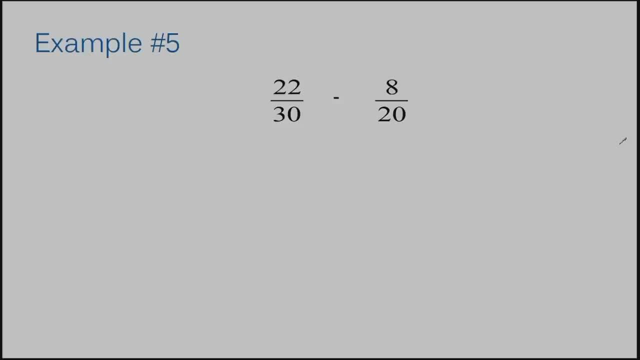 We have a 30 and we have a 20. Many times when finding a common denominator, you're going to have to solve for the least common multiple. We use the least common multiple to become our denominator. 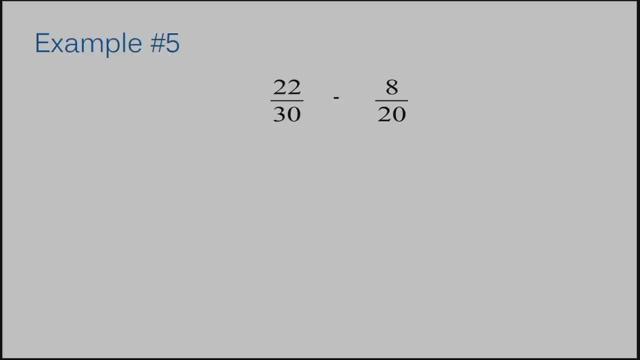 If you're not familiar with how to find least common multiple, you can check out my least common multiple video. It goes into a whole lot of detail of how to do this. 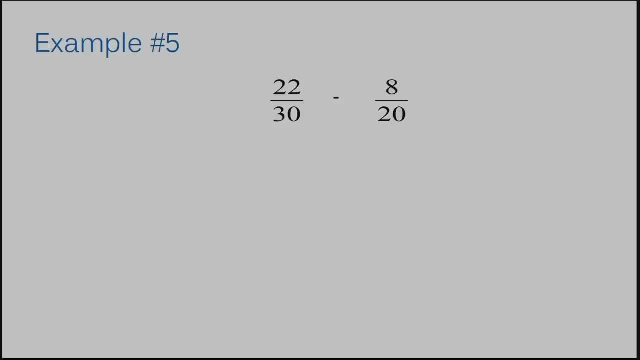 I'm not going to use a lot of time explaining that concept. Because in general... Assuming that you already know how to do it at this stage, I'll just give a kind of brief overview of it. 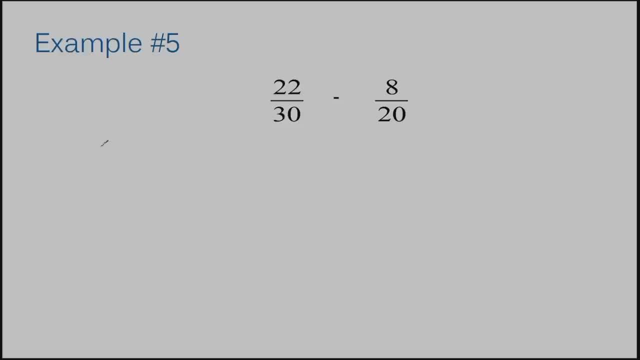 You can basically list your multiples out. I could write 30. Then 60. Then 90. 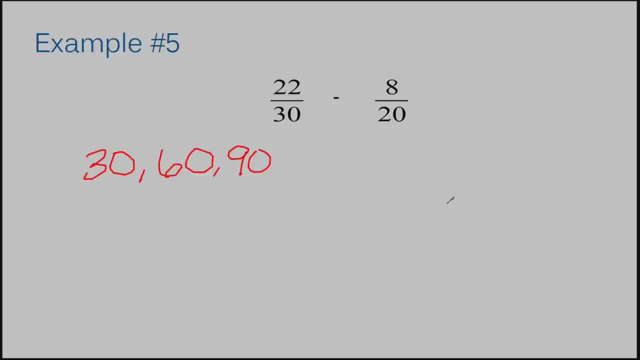 And remember, multiples go on for a long time. So we could write these for a long time. So we're just going to pick a place and stop. 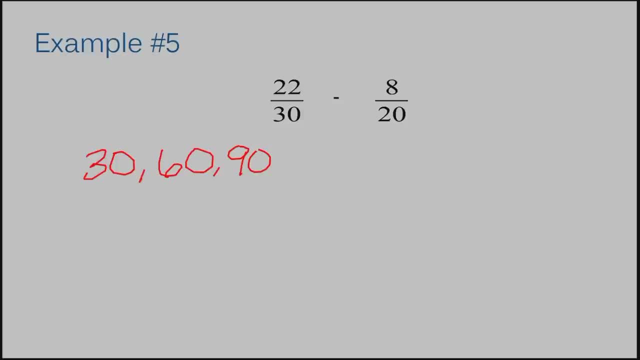 I'm going to list now my multiples of 20. I have 20, 40, and 60. 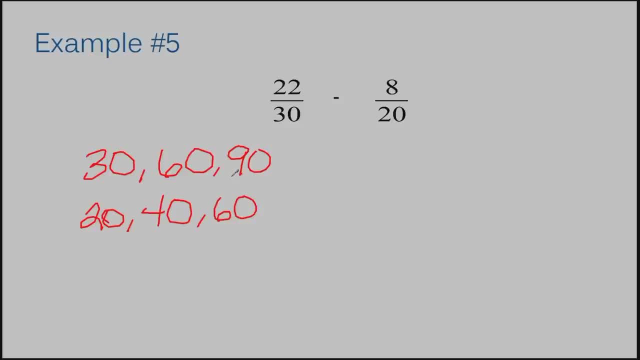 Now when we're finding the least common multiple, that means it's the first number that they have in common. So 60 is the first number that they have in common. So my new denominator is going to be 60. 20 times what gave me 60? 26. 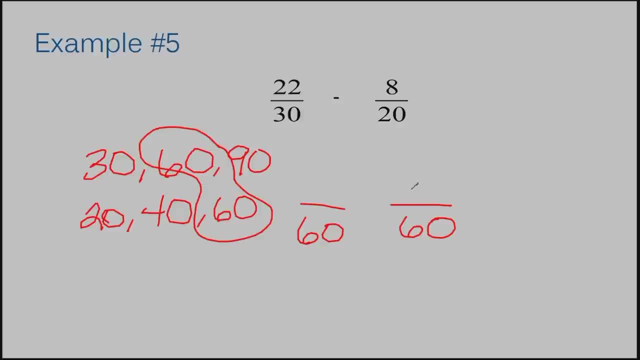 30 times 3. So that means I need to multiply my 8 by 3 also. And that gives me 24. I have to subtract here. 30 times what gives me 60? 30 times 2. So that means I multiply my 22 times 2 as well. And it gives me 44. Now 44 minus 24 is 20. 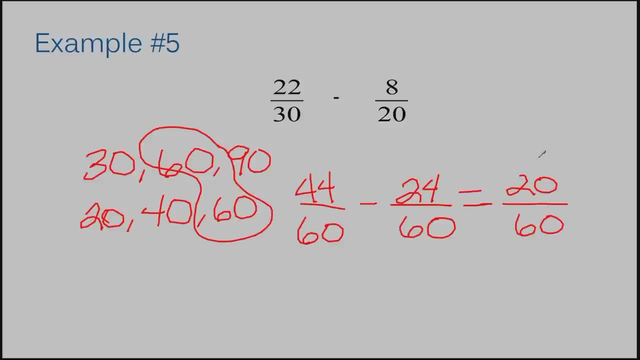 And 60 remains the same. My 0s cross off. And then I can simplify 26. And that becomes 1 third. My final answer for example number 5 is 1 third. That's my last example. Thanks for watching.